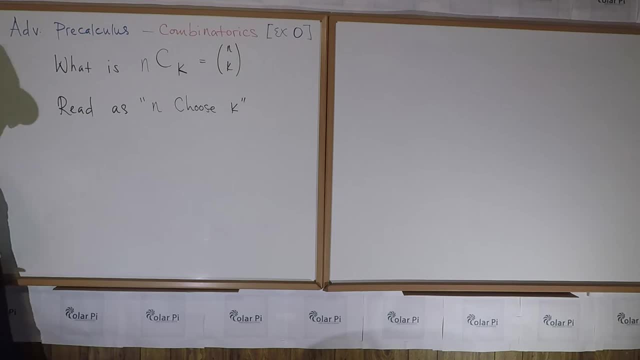 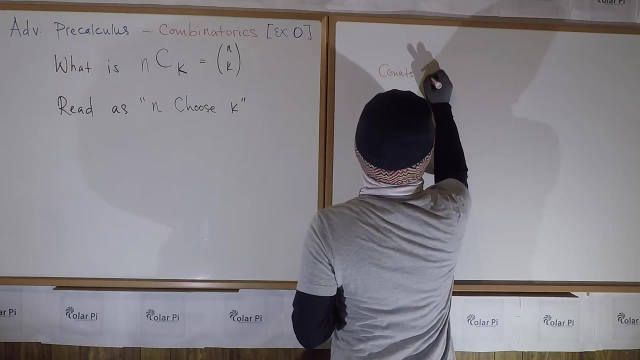 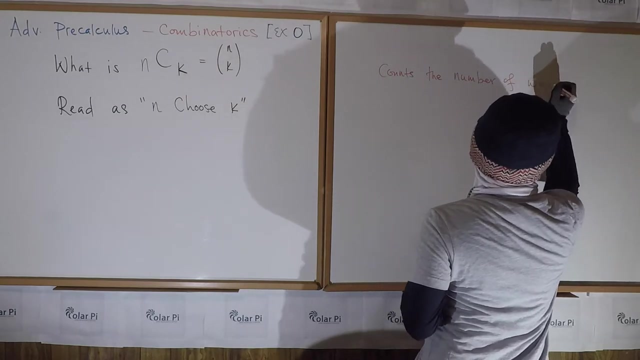 better than me, Okay, anyway. anyway, it's read as and choose K, And what it does is this: It counts, counts, The number of ways And, of course, implicit in this is the number of different ways. right, And? 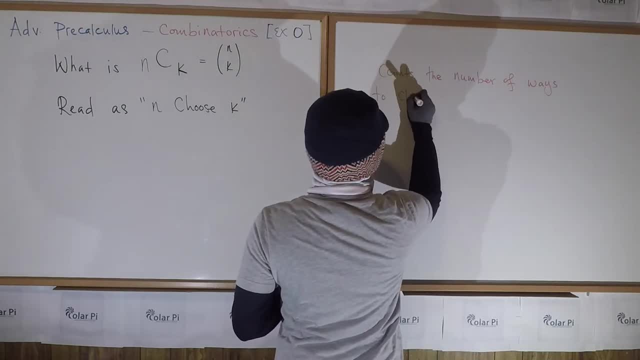 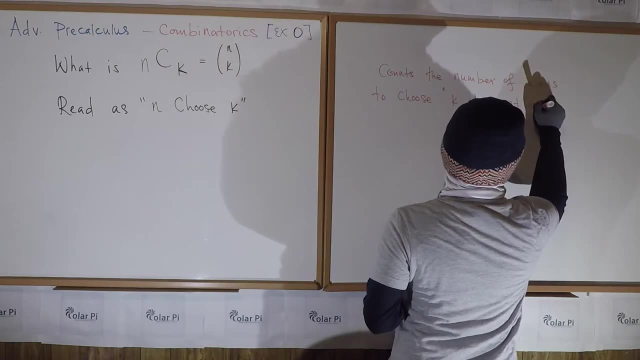 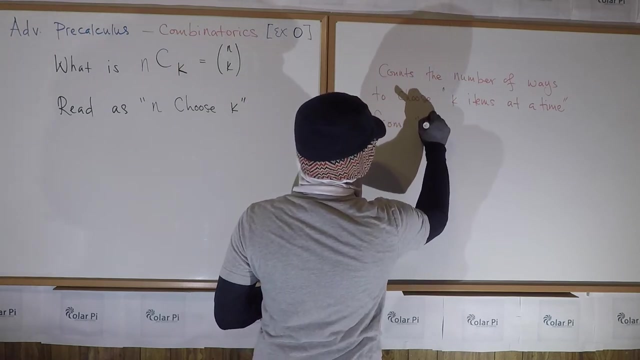 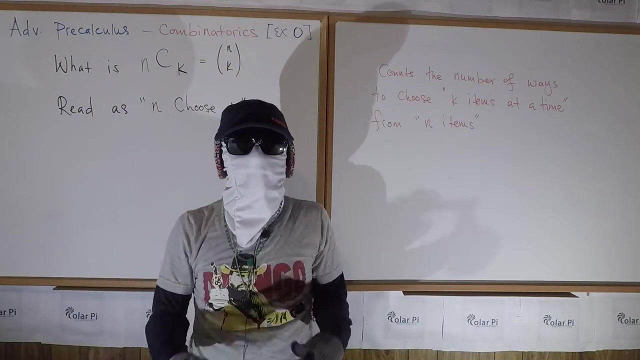 so the number of ways to choose K items at a time from N items. And I'm not being vague when I call them items, because it could be markers, as I'll demonstrate shortly, or it could be dots, as you'll see in example one, But basically all it does is like: 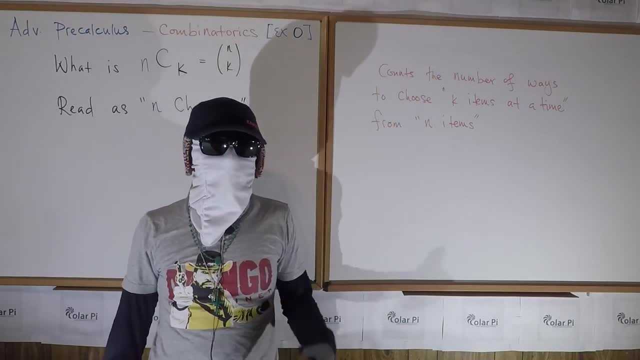 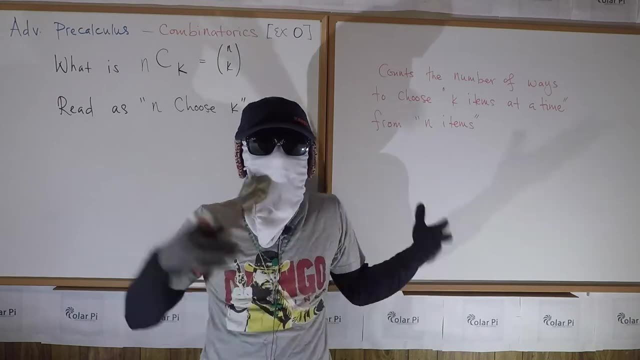 let's say you have like 20 of something and you want to choose like five at a time. Well, there are different combinations of five at a time that you can choose from 20, right? So what N choose K does is it counts the number of different ways to choose five at a time from 20,. 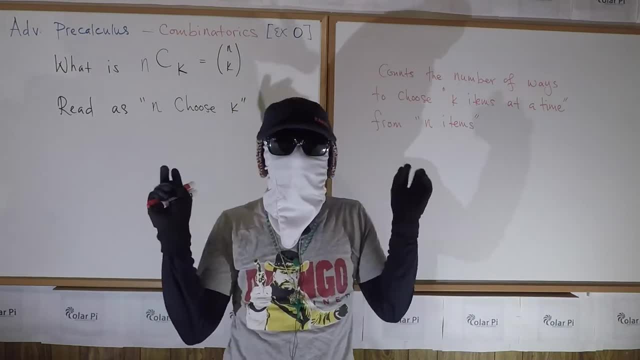 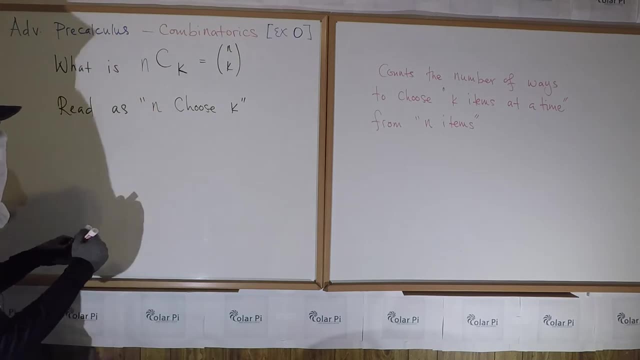 and the example of 23 in the first place. So, and like I said, it counts the number of ways to choose, choose 5, and I'll like give you the formula and like we'll count and stuff. but yeah, first let's do this by definition, right, by definition it must be. 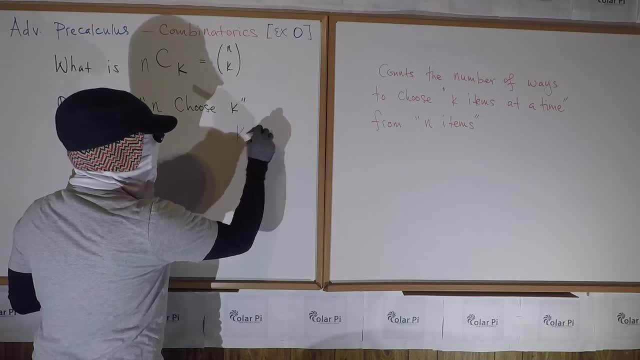 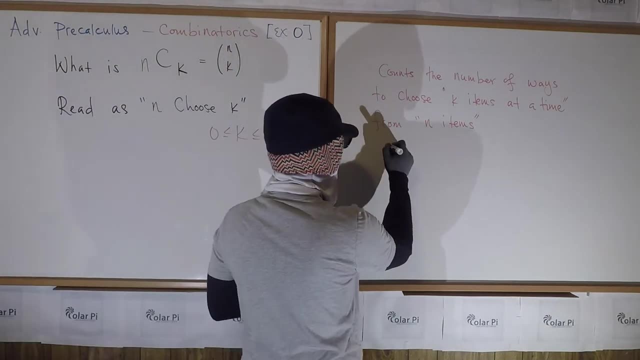 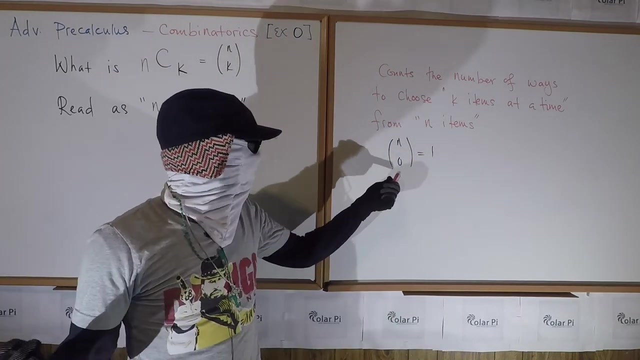 true that K is at most equal to n and at least 0. right, and on this note, while we're at it, let's write these two important results down: which is n: choose 0 is equal to 1, because there's only one way to choose: nothing out of n. 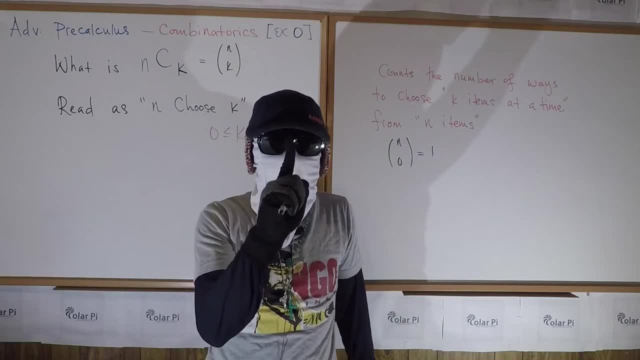 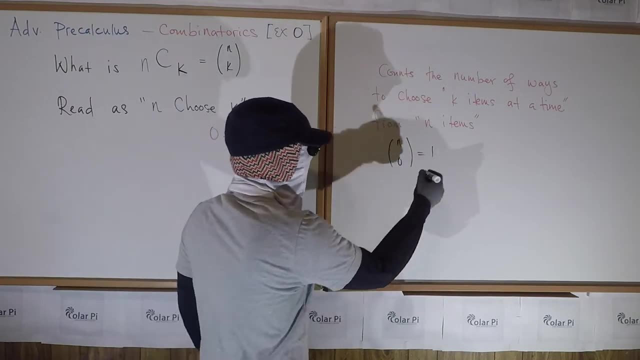 things right, which is you don't choose any of them. there's only one way to choose zero things from n things, and that's to choose none of them. right, and so that's one. also, as you can imagine, and choose n is also 1, and that's. 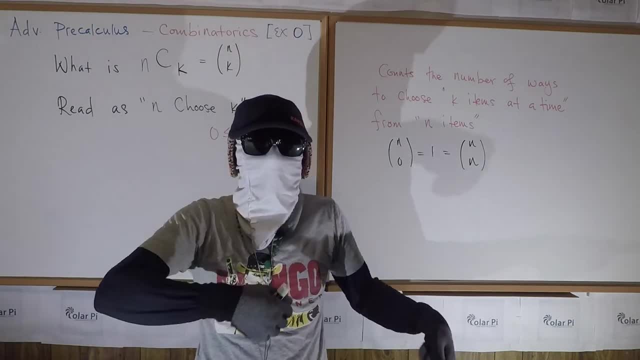 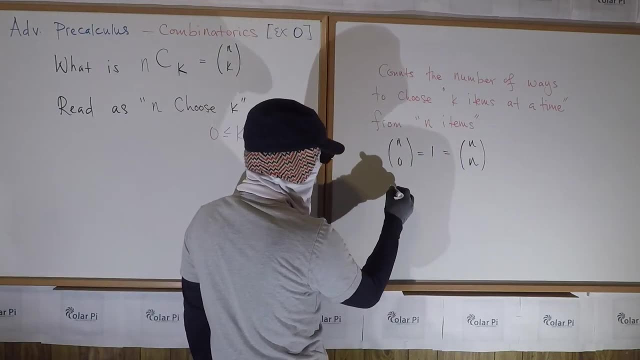 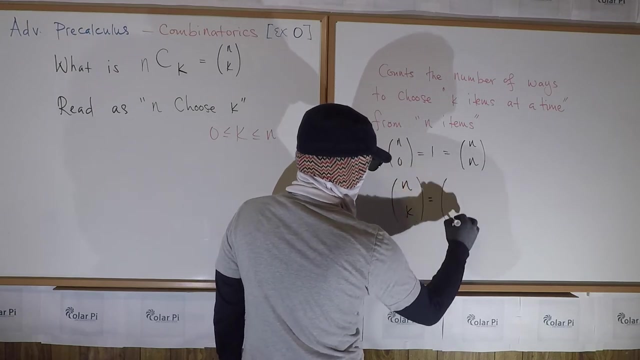 because the number of ways to choose n items at a time from n things is 1, you choose all of them, right, okay, okay, and perhaps we'll dedicate a video to this other result. but it also turns out that n? n choose k is the same as n choose n minus k. 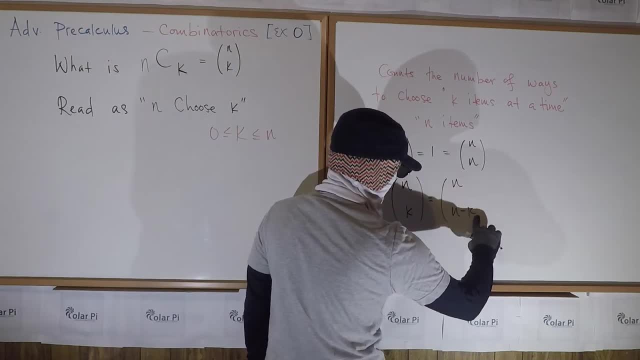 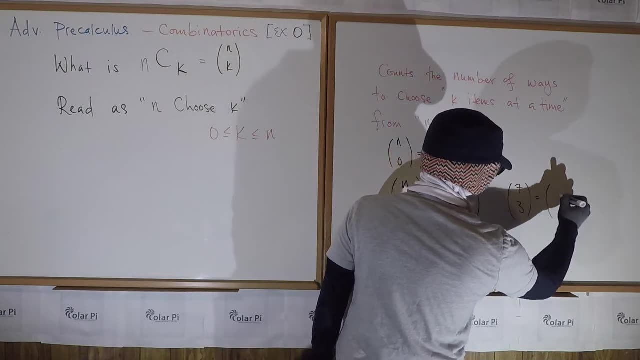 And so, for example, we're saying here: ah, I don't like my writing. We're saying here that, like, 7 choose 3, 7 choose 3 is equal to 7 choose 4. And it makes intuitive sense. 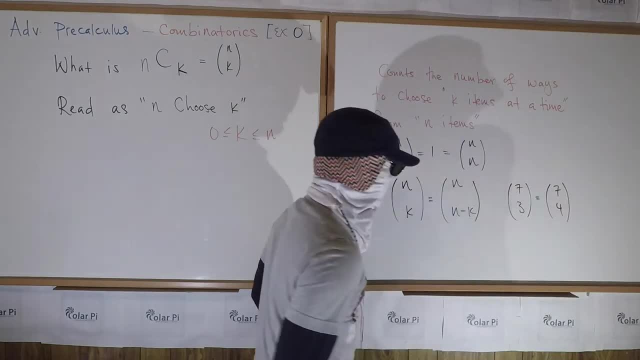 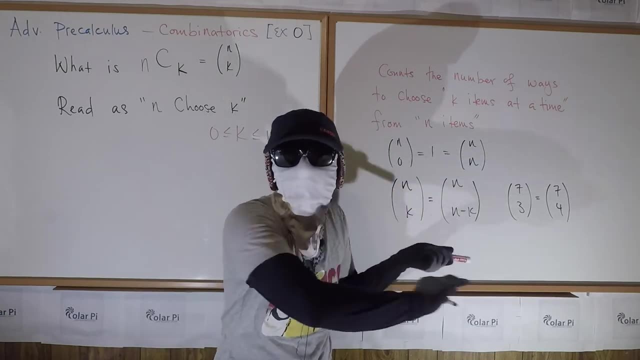 because if you're choosing 3 at a time from 7 items, well, you're automatically choosing 4 items at a time and the 4 that you're leaving behind. So that's why this is true And I don't know that it merits a different video. 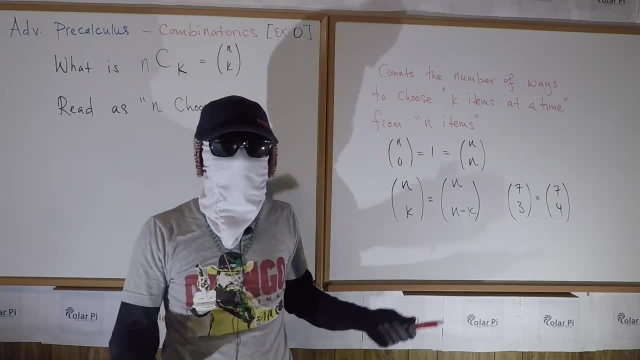 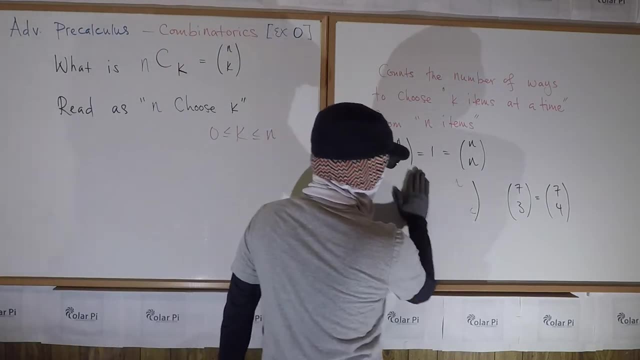 because, yeah, like I hope you get it And if not, then ask questions in the comments section and I'll be happy to help you. Yeah, Okay, okay, okay, All right. so with these preliminary definitions out of the way, 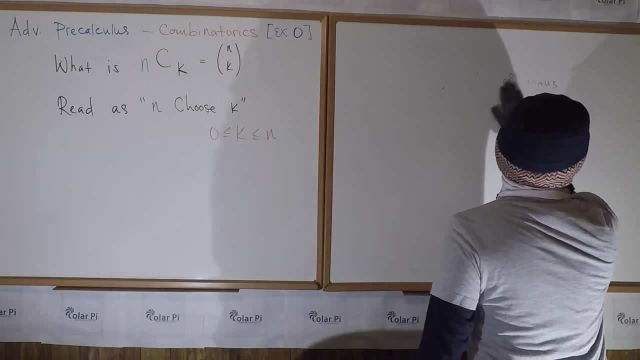 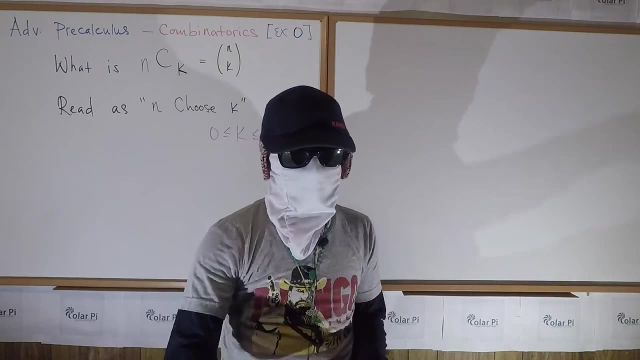 let's actually, like you know, like get more examples, more concrete examples, yeah, Okay, So suppose that what I want to choose is 2 markers at a time from 3 markers, And my 3 markers of choice are red marker, not pen. 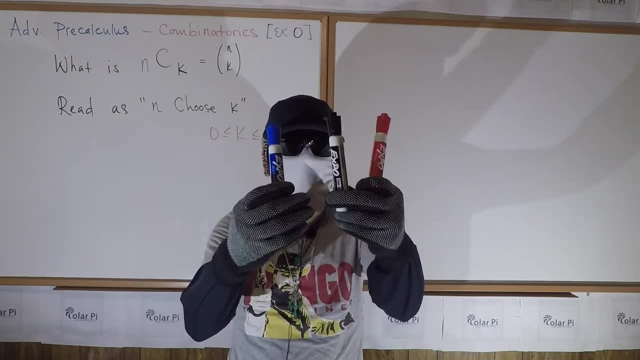 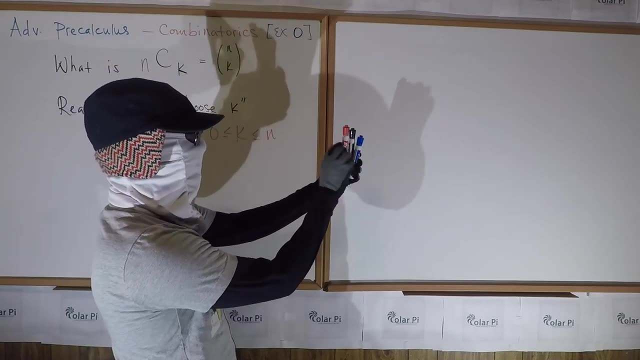 red marker, black marker and blue marker. So I have 3 of these and I want to choose 2 at a time, And so, first, this is what we could do, right? So I have 3 of these guys. 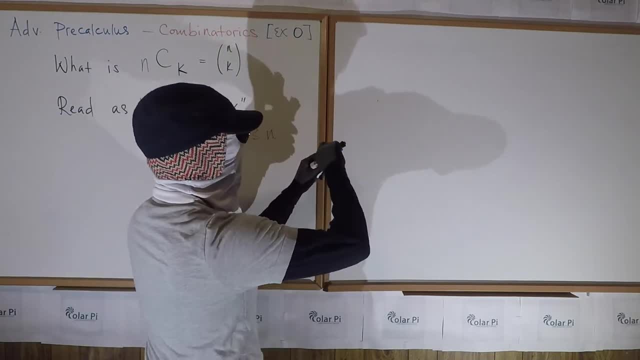 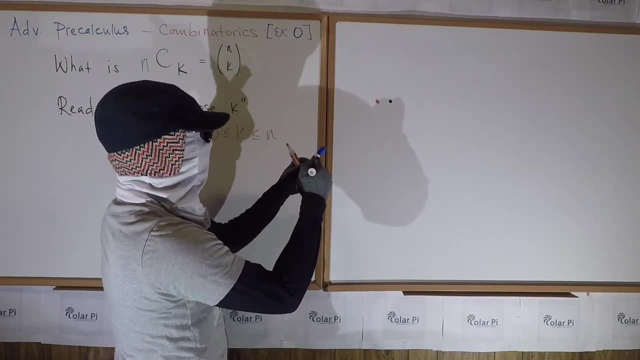 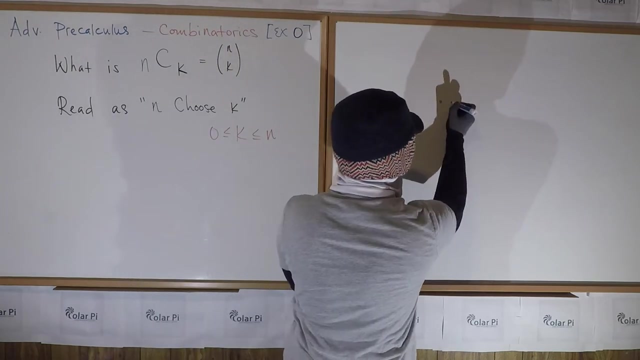 I can choose 2 at a time. right, I can choose red- Let me do that more visibly. I can choose red marker and then black marker, right. Or I could choose red marker and blue marker, right, And what's the only choice, what's the only combination I haven't done? 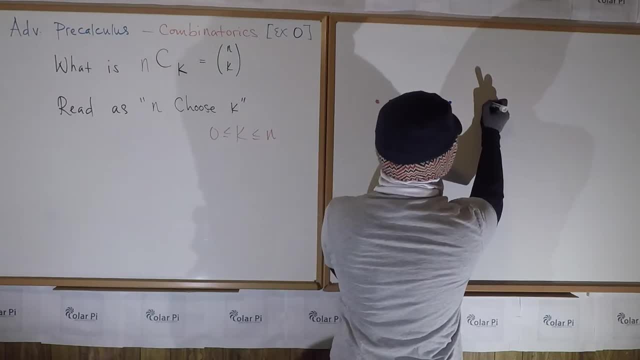 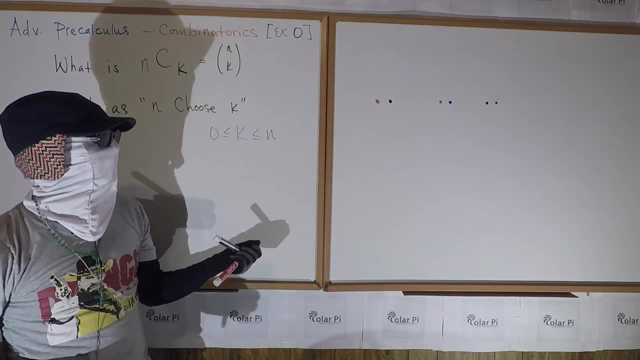 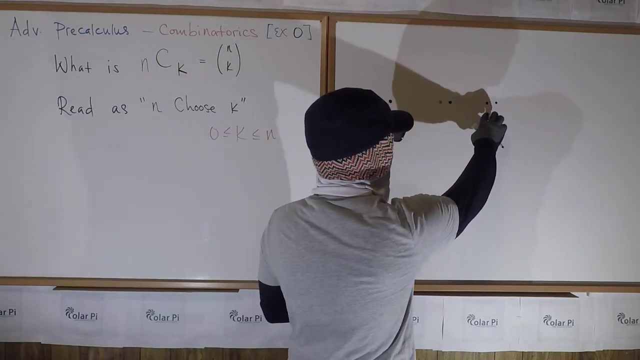 The only combination I haven't done is black marker and blue marker, right, And so you see that there are 3 ways to choose 2 at a time from 3 items, right, And notice, the order doesn't matter. I didn't list like blue marker and black marker as a new separate addition, right. 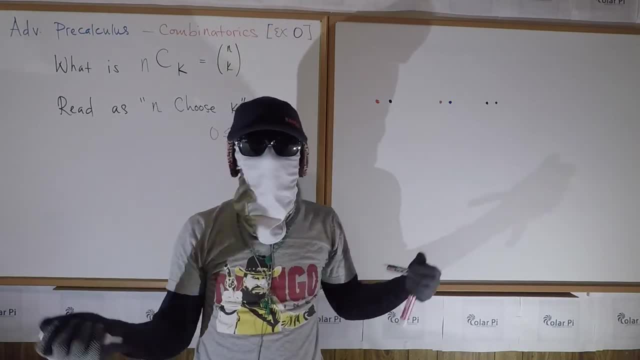 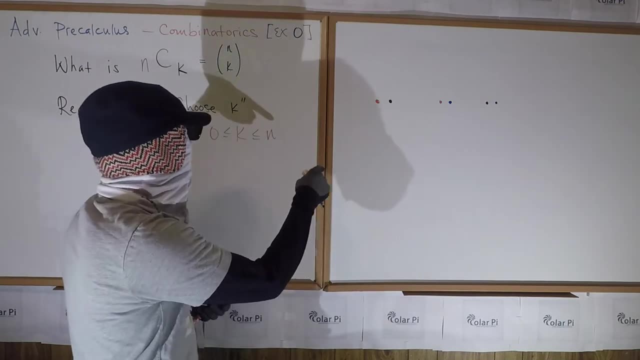 Like this, black marker and blue marker is the same as blue marker and black marker. That is order doesn't matter. You're just trying to figure out how to pick 2 at a time from 3 things, And so what we'd say in this case? seeing the result, 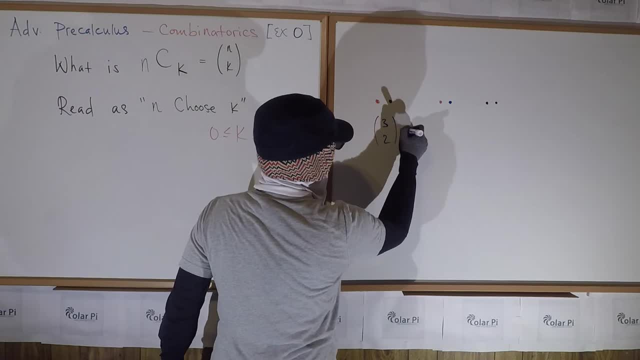 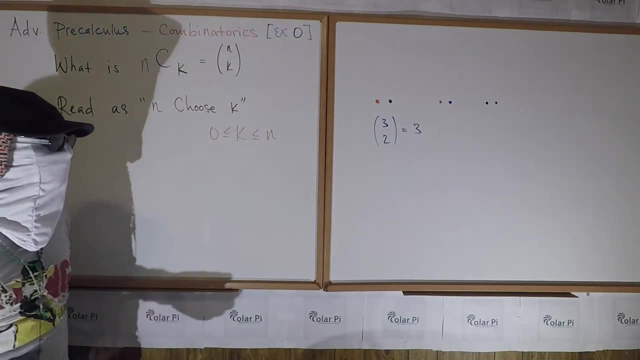 is that, like 3, choose 2 is equal to 3.. The number of ways to choose 2 at a time from 3 things is 3,. right there, Okay, At least with this example. right, Okay, okay, okay. 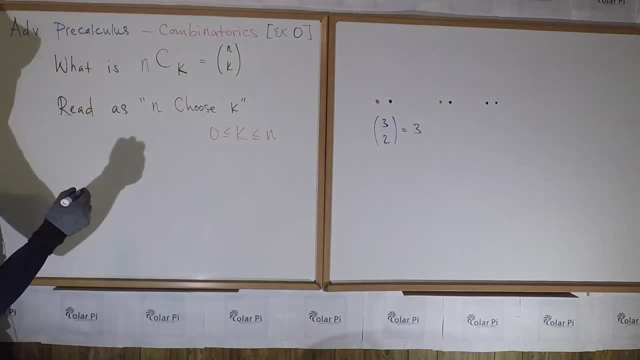 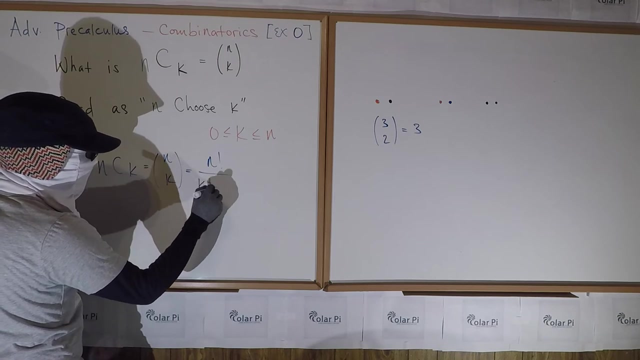 And so so. so, so like, let's use the formula. Okay, so the formula is this, which is: n choose k, n choose k in either denotion right is equal to it's equal to n factorial divided by k factorial times n minus k factorial. 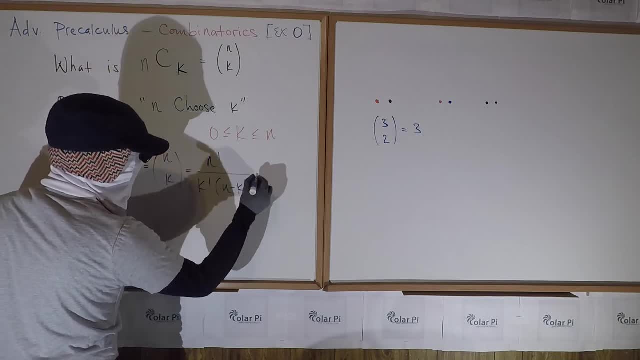 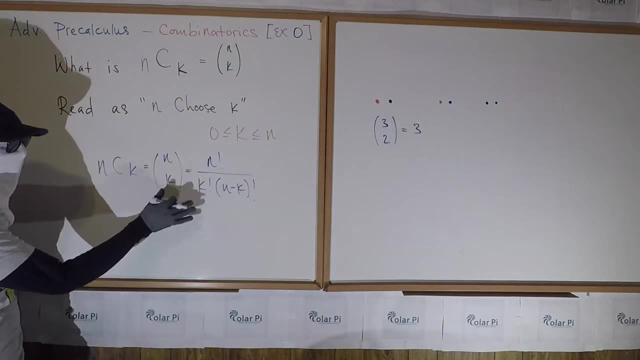 So this comes up so frequently- including, you know, prominently, Prominently, featuring in the binomial expansion formula and the like- that I would commit this to memory. It comes up frequently in probability also, And so if you're a high school student or a college student, 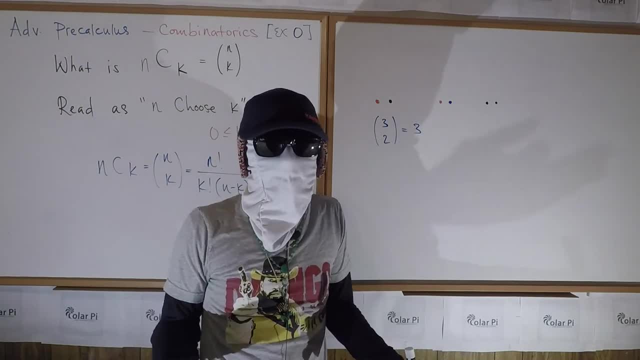 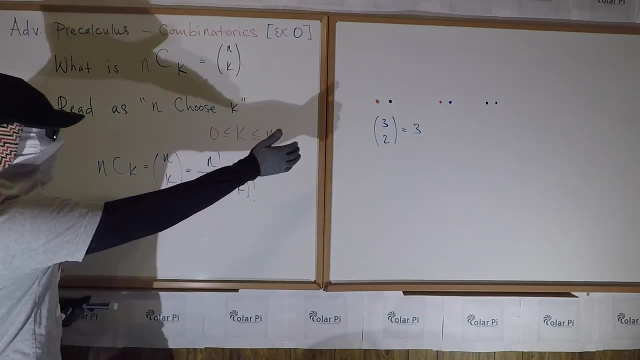 this is really worth remembering, as opposed to you know some random like fact that you choose to remember that I probably can't care less about. yeah, Okay, now let's use the formula to see if, in fact, 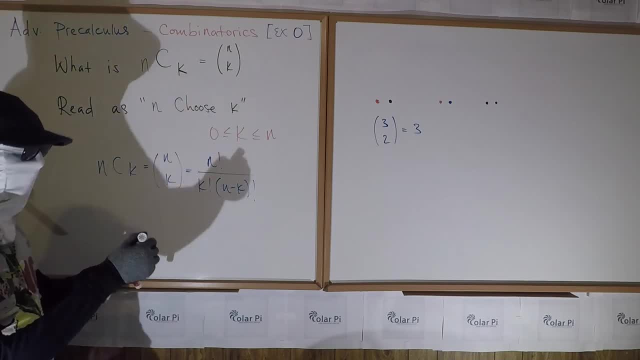 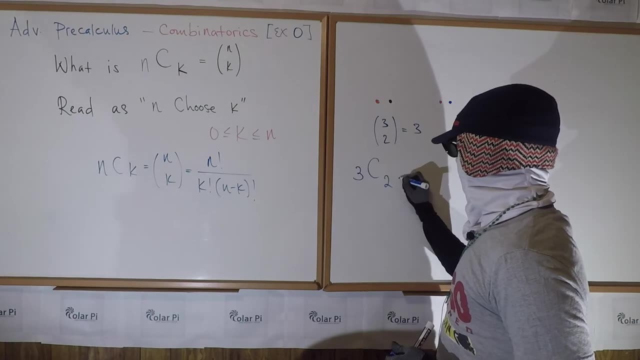 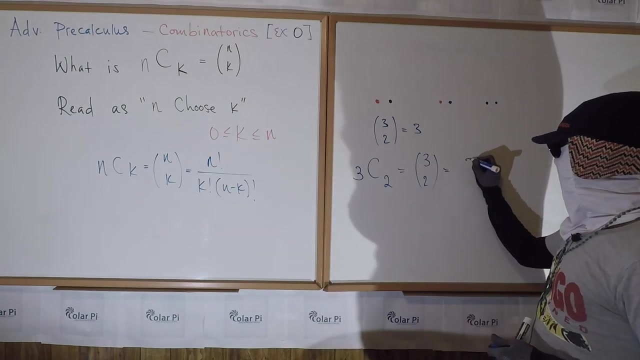 3 choose 2 is 3, as we claim that, yeah, Okay, so it's 3 choose 2, 3.. So we'd write 3 choose 2, or like this: 3 choose 2.. And either way the formula says n is 3,, so that'd be 3 factorial. 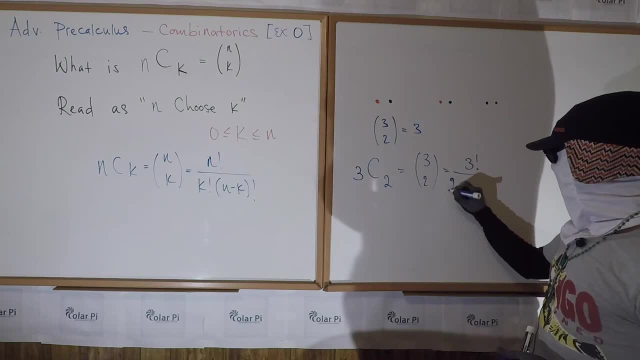 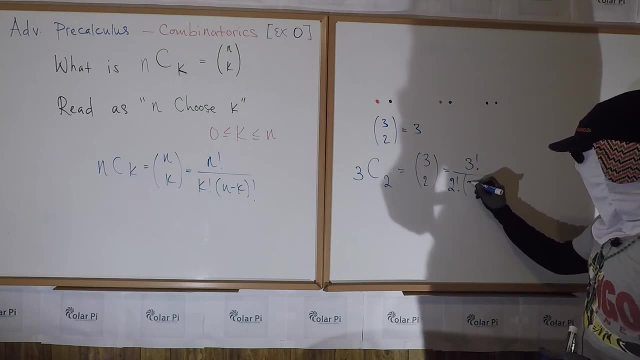 And then k is clearly 2, so divided by 2 factorial times 3 minus 2 factorial. Ah, this blue marker: 3 minus 2 factorial, like that right Okay so. so, so would would it be 3 minus 2 factorial. 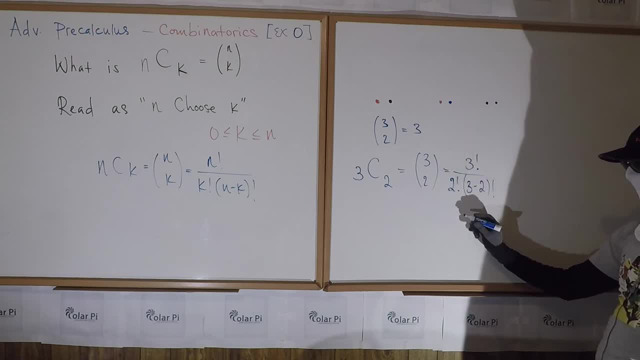 Okay, so. so so would would it be 3 minus 2 factorial. What would that be? That'd be like: well, 3 factorial is 6, so it'd be like 6 divided by. 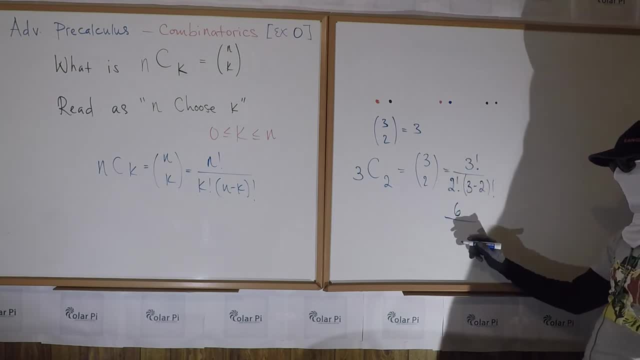 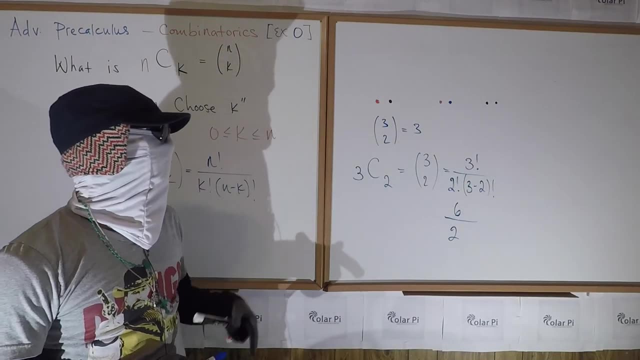 and this is 2, and that's 1,, 1 factorial, which is the same as 1.. So 6 divided by 2, and that in fact is 3.. So, obviously, like you know, if the number of items you have is like, 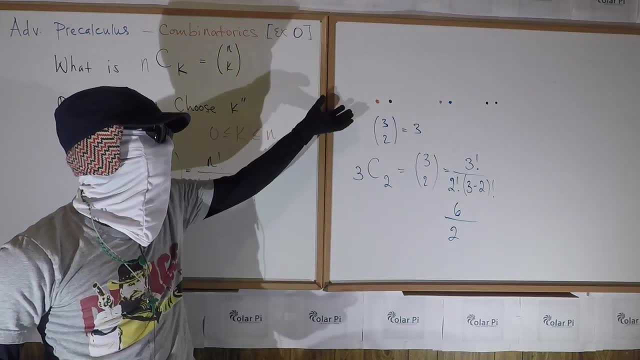 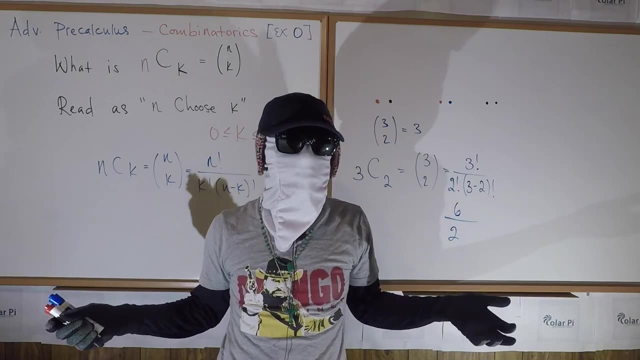 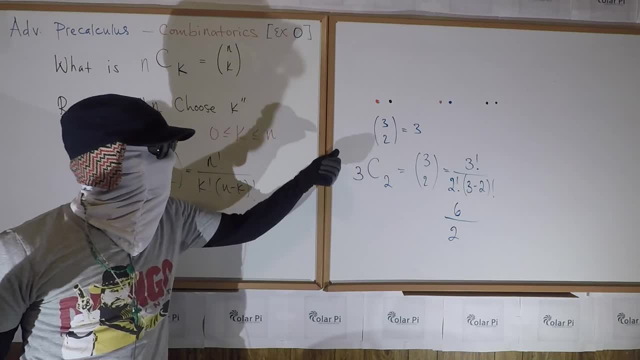 how many different ways there there is. to choose 11 of them, then I'd probably want to use uh, this formula right, And so that's where it's handy.